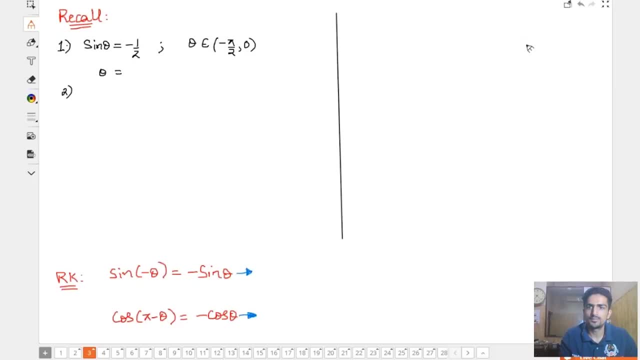 Kindly focus on this thing. You got to tell me theta here. Very good, very good, very good. Siddharth, recheck. Bhakti Niyantra, I couldn't read your. maybe I missed it. Beta, whoever name I'm not taking, they are right. 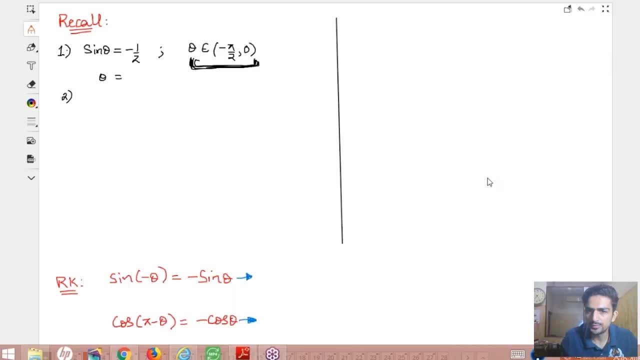 Okay, now Stop. Now stop. More than half of you were wrong, not because they are telling the wrong value, but they are not focusing here. I said: tell me that theta. it lies in minus pi by 2 to 0.. 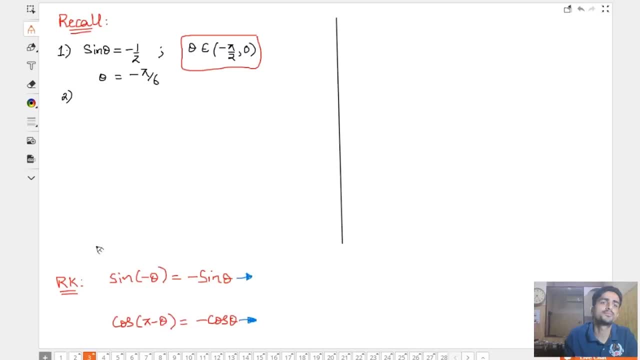 Answer is minus 0.. It's pi by 6.. Sine, theta is minus half for many values of theta, obviously, But I said I need theta in minus pi by 2 to 0.. Okay, I'll give you one more chance. 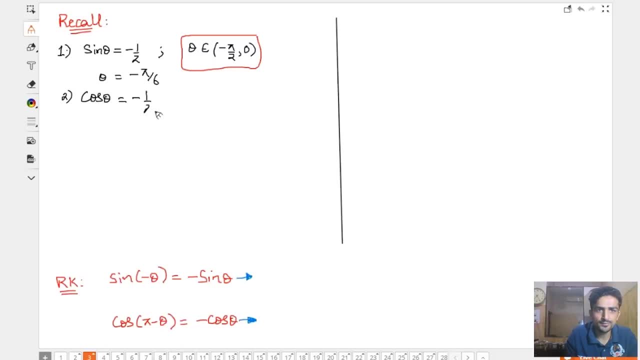 Cos theta is minus half. Theta lies in pi by 2 to pi. What should be theta? Are you sure I could see that beta? Now you tell me your answers. Okay, now you guys stop Everybody. no more message now. 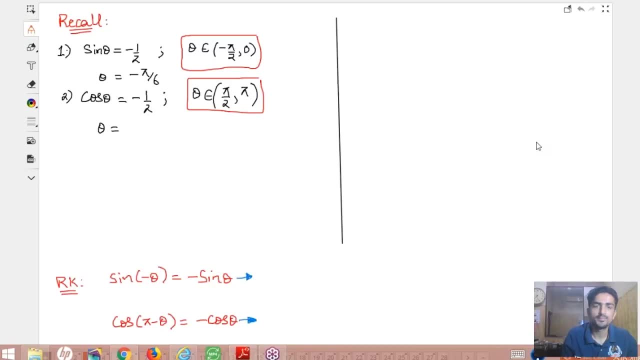 Stop. Still, I don't know what to say. Still, about 7 to 8 students didn't notice this. They are telling me theta, which doesn't lie in pi. by 2 to pi. Somebody is saying minus something, Somebody is saying more than pi. 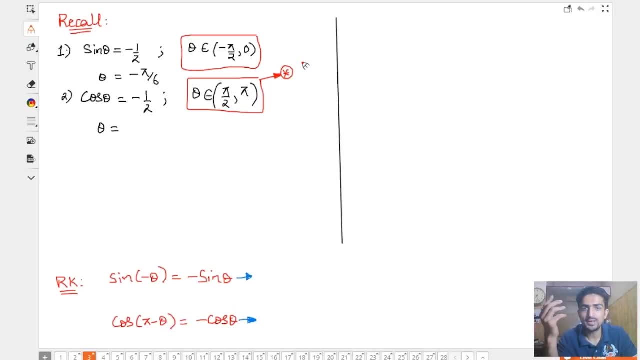 Somebody is saying pi by 3.. Beta, at least look here, Beta, you cannot miss it twice. Even initial question, I put stress here. Now again you are not looking at that. Somebody is saying minus pi by 3.. 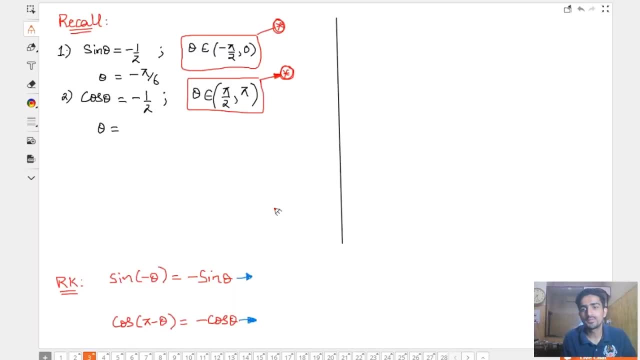 Beta does minus pi by 3, lies in pi by 2 to pi. Which math do you study, beta? Okay, So first of all, answer is 2 pi by 3.. Yes, Shagun, that is the problem. 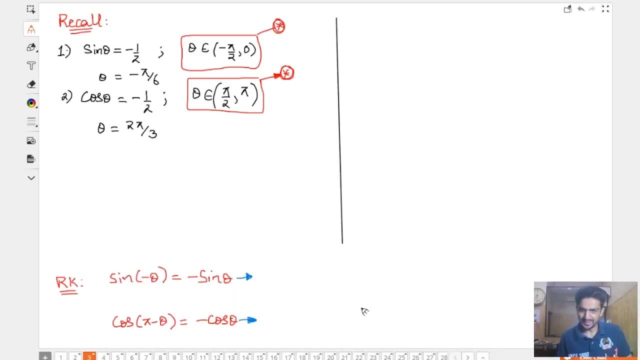 Because basic questions. still, you are giving wrong answers, And that is quite common, Don't you worry about that? That is why I am revising it. Okay, wait, wait, wait, wait a bit. My purpose is not to like, just make you uneasy. 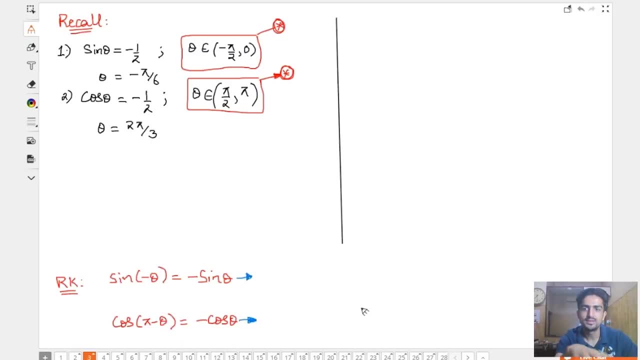 My purpose is to make you realize that this is required. This is something Many of you- many of you- are not good at or they have forgotten it. Okay, Before proceeding ahead, let me just revise it first. now Look, guys, for sine. keep this thing in mind. 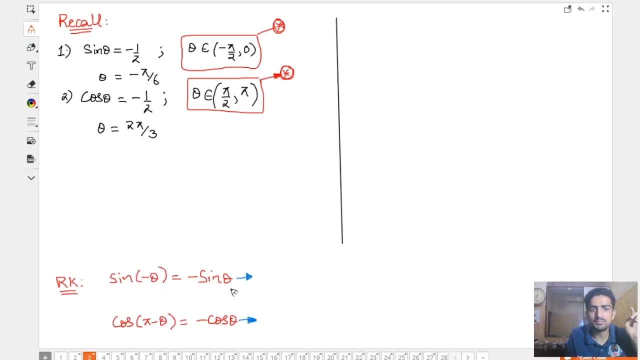 Sine of minus theta is minus sine theta, That is. let me explain it through an example. We know sine of pi by six is half. If you don't know even that, you better leave the mathematics. We know sine of pi by six is half. 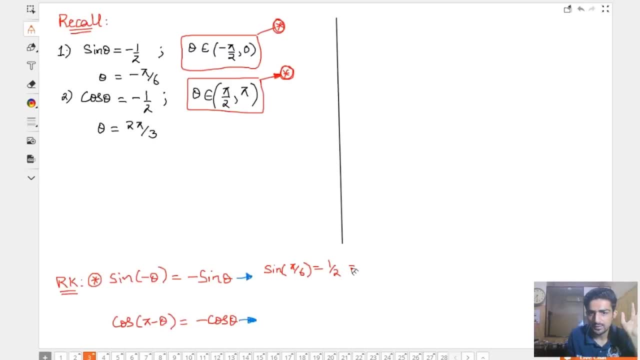 Then this thing tells me that sine of minus pi by six will be minus half. Just relate this result with this example: Sine becomes negative at negative angle. Simple Sine becomes negative at negative angle. If sine of pi by six is half, then sine of minus pi by six will be minus half. 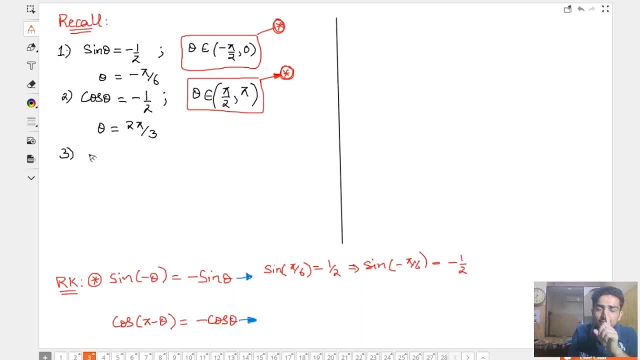 For example. now please nobody message me. if I say sine theta is minus one by root two and I ask you: theta in minus pi by two to zero, then you will think it like this: your sine theta is one by root two at pi by four. 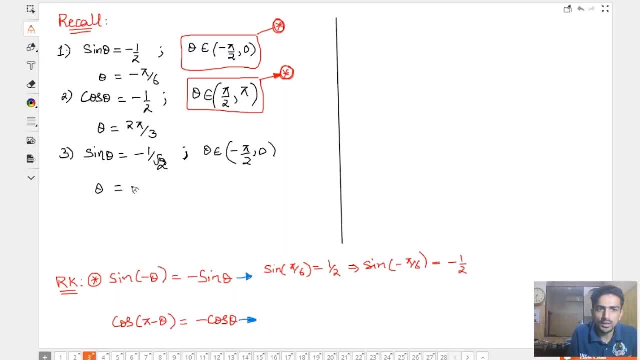 Then it must be minus one by root, two at minus pi by four, because sine becomes negative at negative angle. Now let us talk about cos theta. I hope you understand that theta and pi minus theta, These are supplementary angles because their sum is pi. 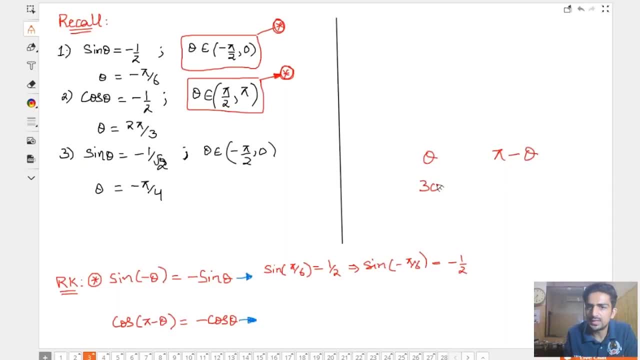 What is a supplementary angle? What is a supplementary angle of thirty degree? It is one fifty degree. What is supplementary angle of pi by three? It is pi minus pi by three, That is two pi by three. These are called supplementary angles. 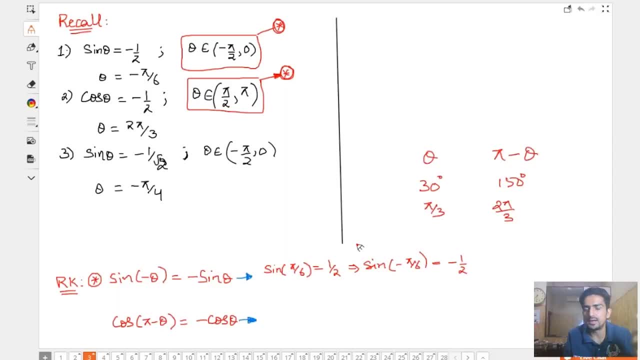 So supplementary angle are the angles whose sum is one eighty. So if I ask you supplementary of thirty, you will tell me one fifty Only. then the sum will be one eighty. If I ask you supplementary of pi by three, you will tell me two, pi by three. 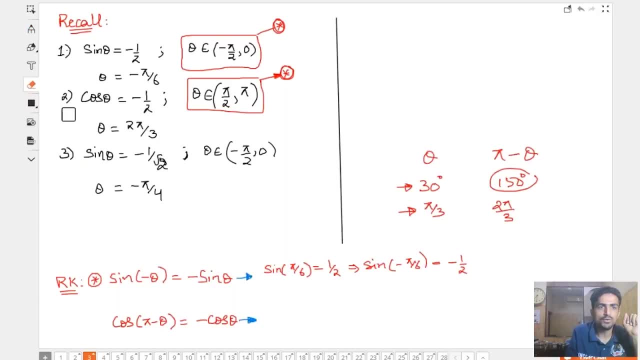 Better wait Now. if you see the result of cos. Cos of pi minus theta is minus cos theta, That is. let me take an example- As cos of pi by three is half, Then this result tells me that if I take supplementary angle I will get negative value. 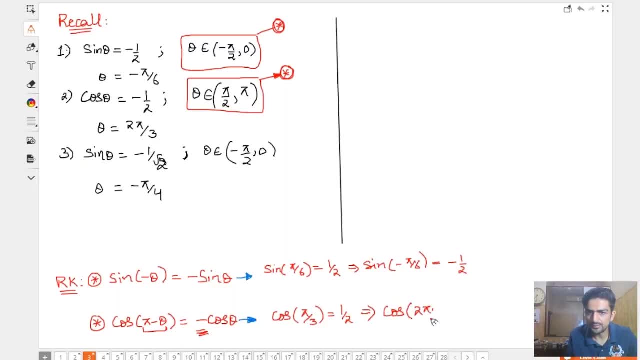 That is cos of two pi by three. Supplementary of pi by three is two pi by three. Their sum is pi. It will be minus half. Cos of pi minus theta is minus cos theta. You need to focus on theta and pi minus theta. 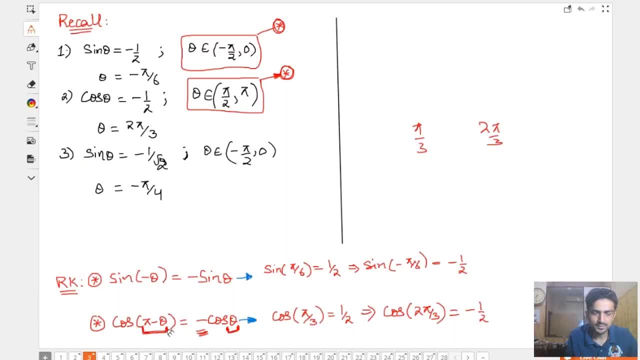 They are supplementary angles, So value of cos at supplementary angles is negative of each other. Let me take one example. For example, if I ask cos, theta has to be minus one by root two And theta should lie in pi by two to pi. 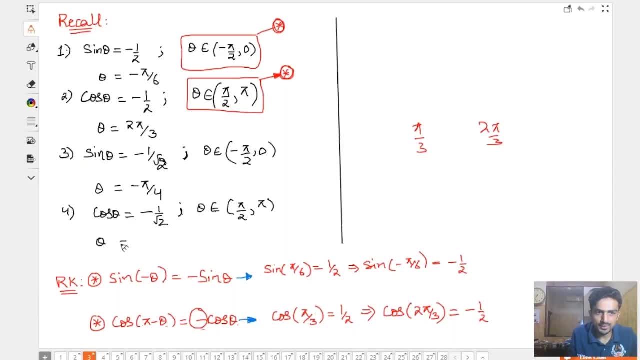 That is second quadrant. Then what will be theta? You will think it like that. You will think: cos theta one by root two. When does it happen Now? cos theta is one by root two at pi by four, Then it will be negative of one by root two at supplementary angle of pi by four. 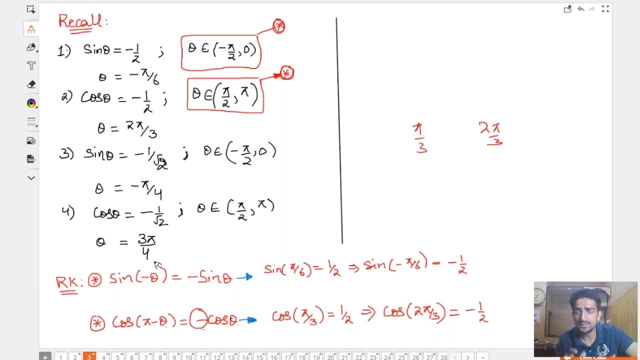 So what is supplementary angle of pi by four? It is three pi by four. Very good guys, Mohithakesh. minus three pi by four, nahin, Three pi by four. What will be the supplementary of pi by four? It will be three pi by four. 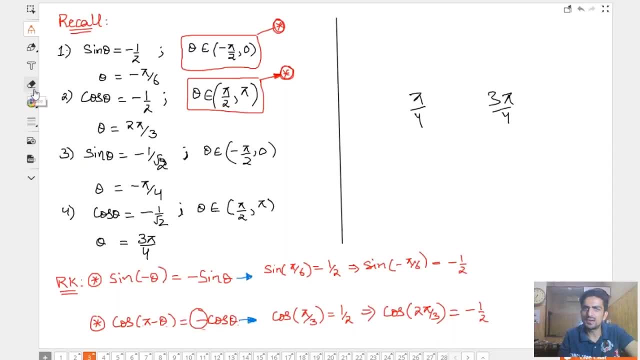 Their sum is pi. It is very easy, because supplementary of pi by four will be pi minus pi by four. This is supplementary angle. no, Now, this is nothing but three pi by four. Okay guys, Now, before I proceed ahead, I give you one complete minute. 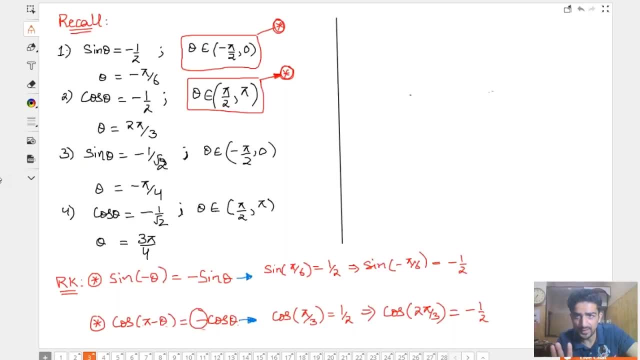 No messages, No doubts. Vivacious wait, I answer to that. No messages, No doubt. Just try to see what I am trying to tell you. Look at these two remarks, Look at these four questions And just try to see what am I trying to explain. 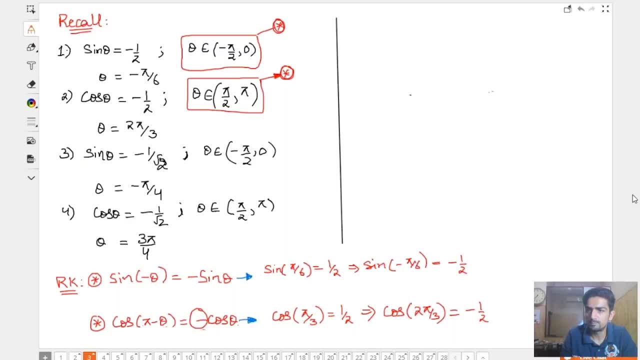 Nothing of this type happens in complementary angle, So we will not use that. Very good, Shantanu. So primarily, I am telling you to find theta when sine or cos are negative. Okay, For sine. you got to remember that sine theta will be negative when theta is negative. 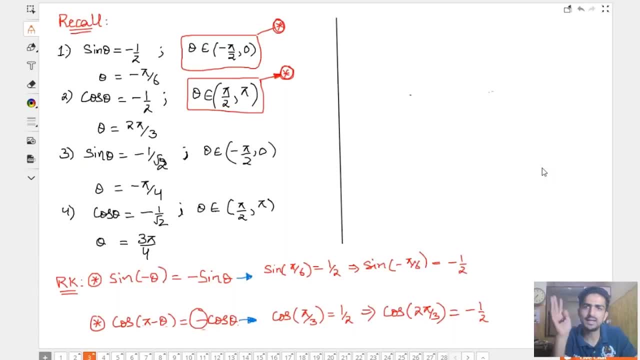 That is minus angle For cos theta. you need to remember Cos theta is negative at supplementary angle. Okay, That is something I am trying to tell you. Many of you might be thinking That, sir, cos theta equal to minus half. It happens at many angles. 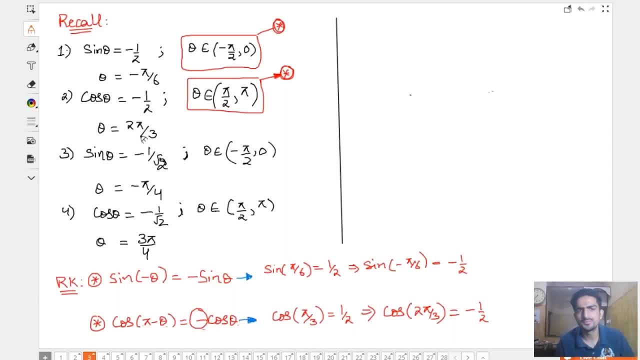 Cos, theta becomes equal to minus half at many angles. But believe me, In this chapter we will be requiring such value And for such values. you got to keep these two remarks in your mind. That's it. Okay, So not at all bad. 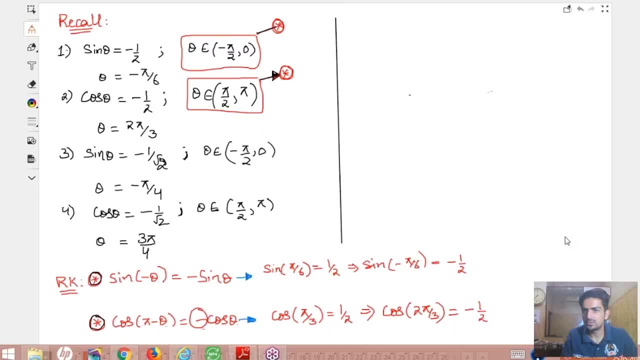 Almost everyone got it. About two to three students have doubts. Let us hope with coming examples it will also get cleared. Yes, Its weightage in JEE main set advance is quite low. Normally direct question comes like in advance. It gets used in some questions. 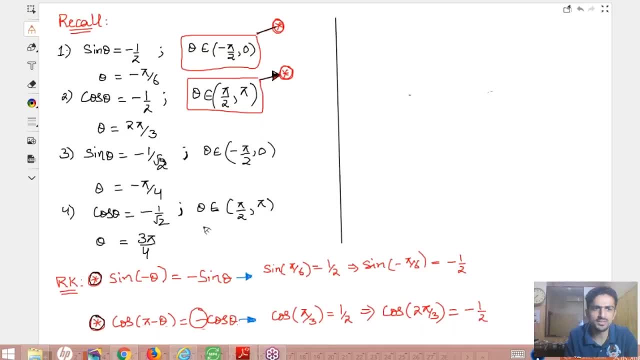 Direct questions are rarely asked on this chapter. Okay, Let me take few more examples. First of all, Guys, Tan and cosecant also have same behavior as of sine. Same behavior That is, tan of minus theta Will be minus tan theta. 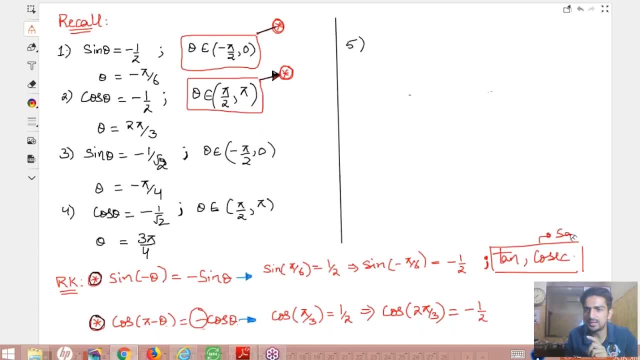 theta Cosecant of minus theta will be minus cosecant theta And the other two cot theta, secant theta. They behave same as that of cos, That is, they will be negative at supplementary angles. So the question is, when I ask you to respond, only then you respond, okay, So that I 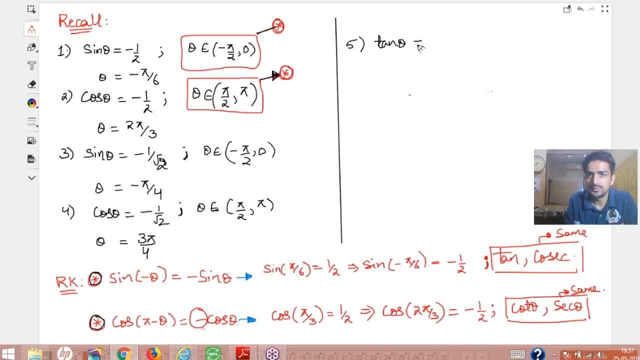 may read the messages. Do not start responding immediately. 10 theta is minus root 3. And theta lies in minus pi by 2 to 0.. You need to tell me theta Now start. Very good, Very good, Very good. 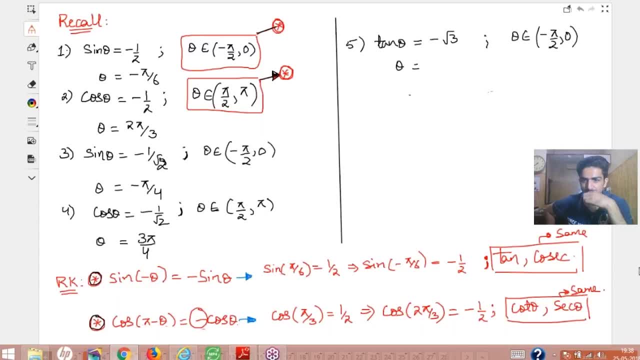 guys. Now you are on the right track. Very good, Nikhil, you took the wrong angle. Idea is right. Very good, Very good. Yes, yes, yes, Very good. Nice Dhruv beta. I will come to that also. Dhruv, you are right, I will come to that also. 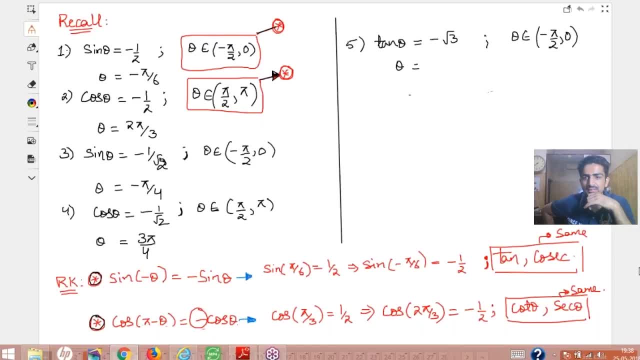 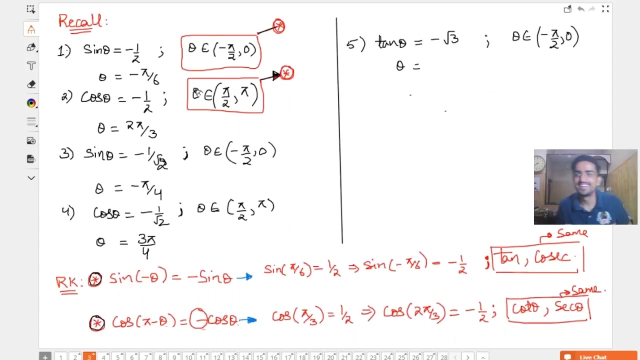 Yes, Shagun Nirav, take care of the angle. beta Idea is right, but angle is wrong. Yes, they are sure. Okay now, stop, Stop, stop, stop, Stop. now, 10 theta is root 3 at pi by 3.. So it will be minus root 3 at minus pi by 3.. 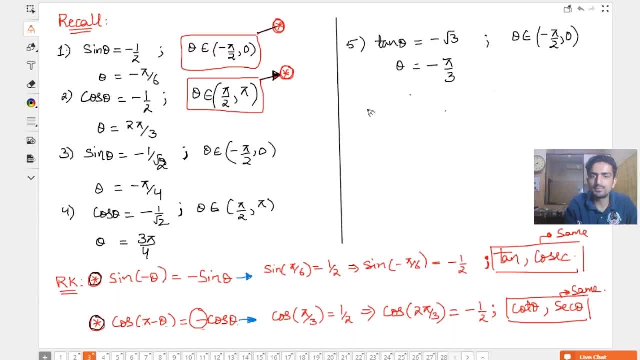 Now, before I give you next example, I just told you cot of pi minus theta is minus cot theta, That is, cot also behaves like cos Somebody just asked. I forgot the name- that's a cot of minus theta is also minus cot theta. Yes, 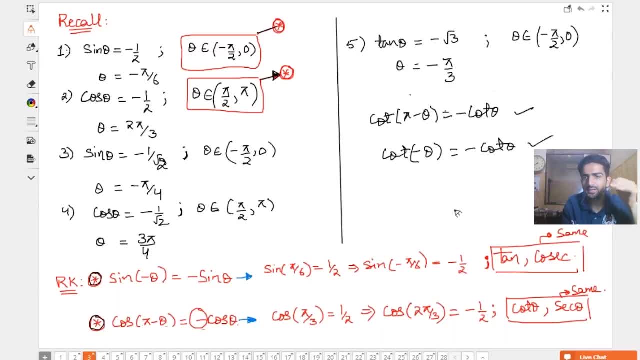 perfect. Both are correct, But in this chapter we will be requiring this thing. Okay, understand why I said so. So in this chapter we'll be finding such questions about cot using this and not this. It will not be useful for us in this chapter, You will understand. 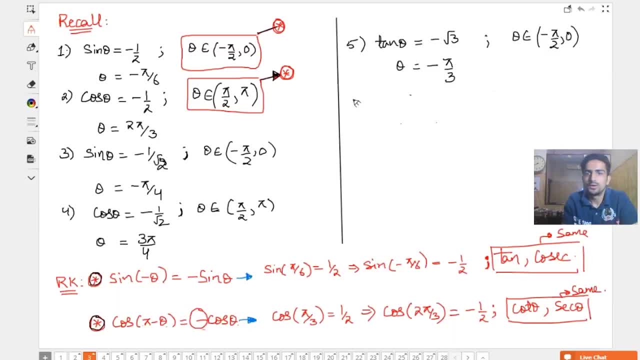 what do I mean by that? So my next question is about cot. only Be careful about angle. Okay, Cot, theta is minus 1.. Theta lies in pi by 2 to pi Shagon. that is Okay. now tell me theta. 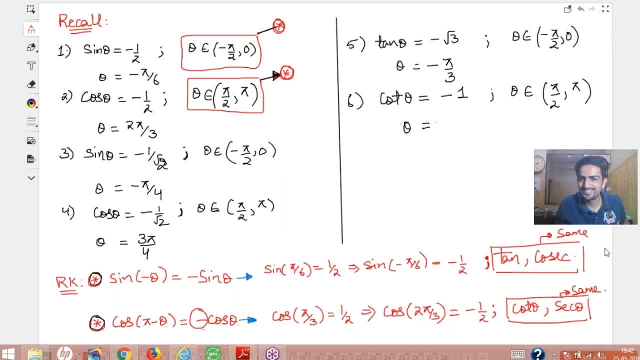 Menak. I can do that. Don't worry, Devya, that is completely wrong beta, Dhruv. if required, I will do that. Nayan, that is wrong beta. How come negative answer beta? Okay, that is fine, Shagon, it's okay beta. Do it, I'll tell you. 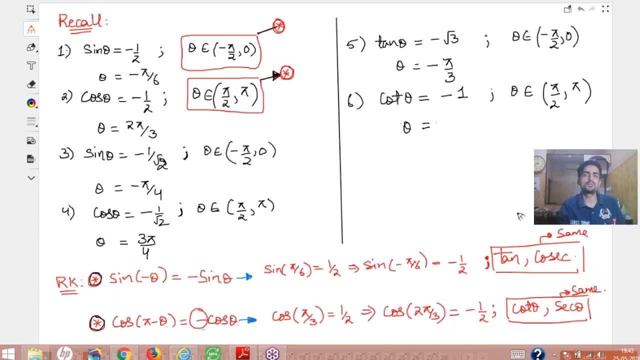 okay guys, now you stop. stop, stop, now, everybody stop. most of you were correct and i'm happy about that. chord theta is 1 at pi by 4, so it will be minus 1 at supplementary angle, which is 3 pi by 4. okay guys, so that is sufficient for the starting. my first two lectures will be like using these: 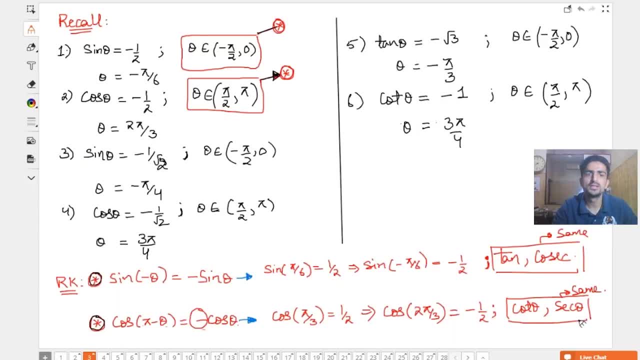 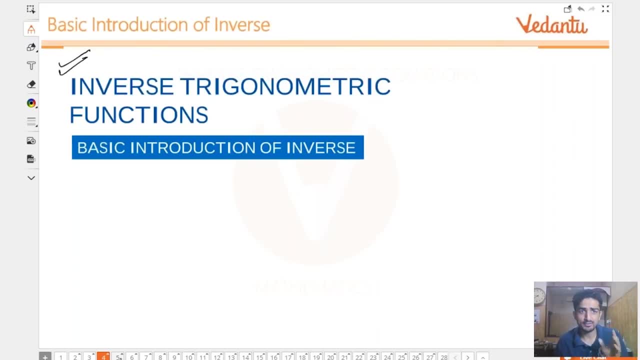 informations. primarily, second lecture will use this information, so i'm happy now you are comfortable with that. let us start with the chapter now. inverse trigonometric functions: uh, first of all, obviously, in this chapter, uh, you, we will study inverse functions of trigonometric functions. that is something we'll be doing in this chapter. 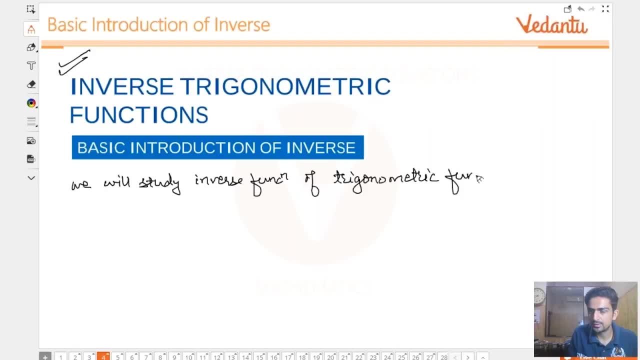 okay, uh, so we know what is inverse of a function backtracking, nothing more than that. now we know, uh, functions are invertible only when they are bijective. we know that. but talking about sine x from real to real, it is clearly not bijective. first of all, let me just discuss uh onto. 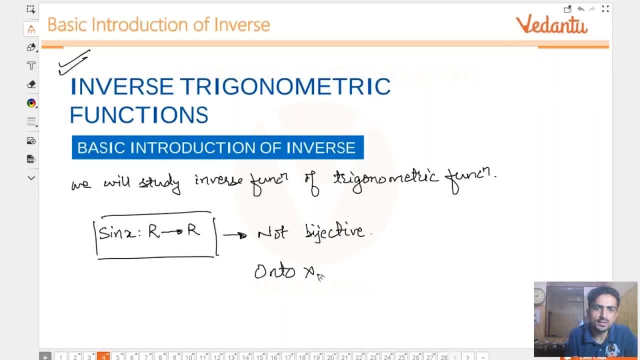 okay, it is not onto, because range of sine x is minus 1 to 1, whereas my co-domain here is real, so it is not onto. similarly, we know the graph of sine x. it is many to one. then clearly we cannot find their inverse. okay, so chapter is finished. their inverses are not possible. go home, enjoy. 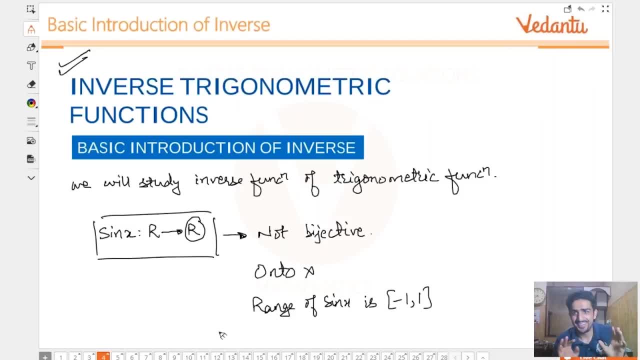 uh, but that is something we cannot do. i wish i could do that. okay, uh, listen guys. uh, certainly, we need to modify them so that they become bijective and hence invertible. do you understand? if i change this co-domain to minus one to one, then my function becomes onto. 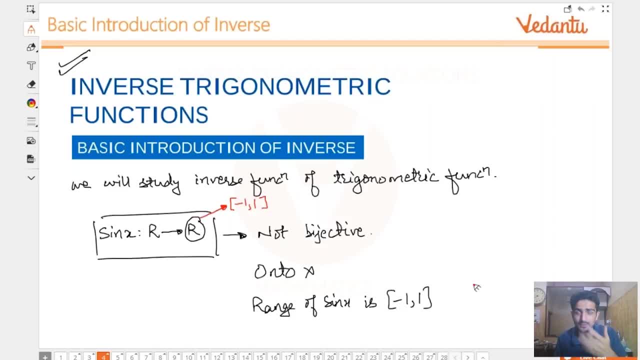 worshiping to do whatever we want, but asucks is optimal. very good guys. very good because what you do what you want is for simplicity: studies, podcast, discoveryВот. here you do everything you want, especially every step. that is really problematic to do, because if people stimulate you in trying to aim to edit handwriting, that is the difference. long road for extension. frame of the script. one great advantage of metal setteraa milan, yes as x them simply skippad. if you are terrible at making a copy, travel in your order. any badم skill 是ى. 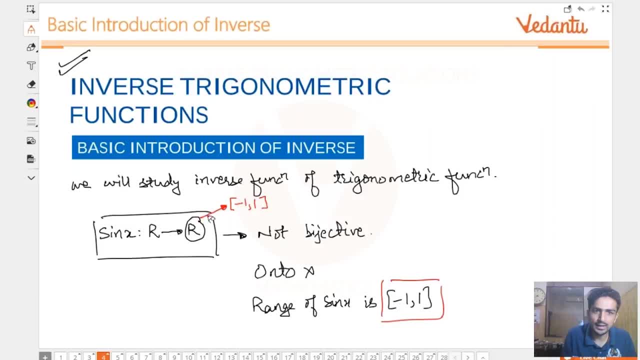 is my range. I took my codeman also to be same. okay, so, similarly changing code, domain or domain, we will try to make it one one and onto, and that new sine X will be invertible and hence we will find its inverse or we will define its. 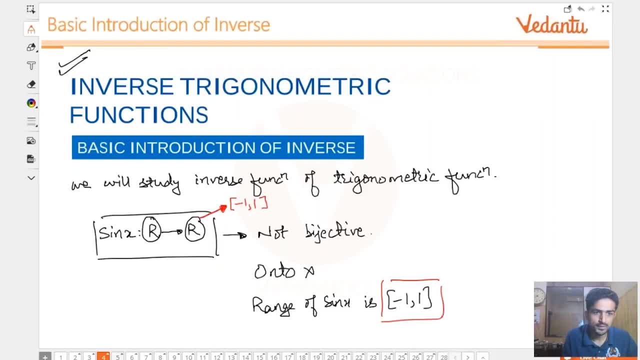 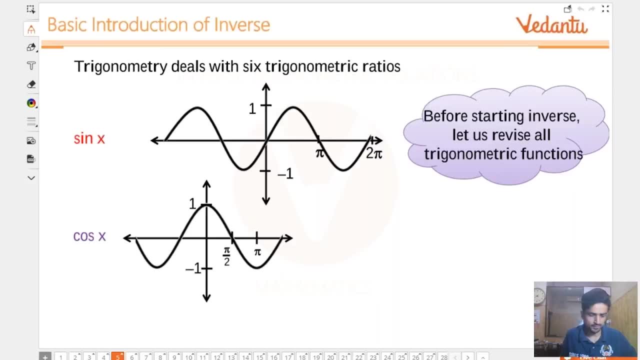 inverse. okay guys, look at the graph of sine X and cos X. those who don't remember, just keep it in mind. I'll not be expecting that you don't remember the graph of sine X and cos X. even so, those who don't remember this, please Abhiyaad. 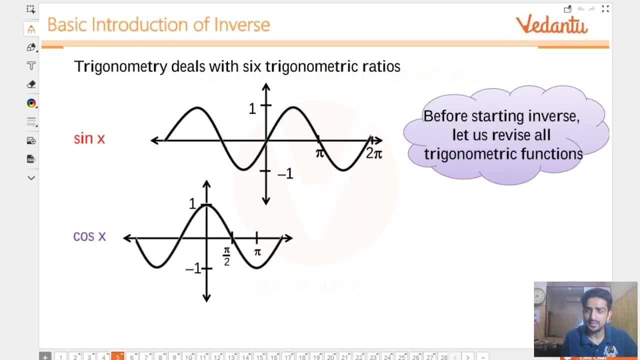 Karlo Karthik, and we can make every function like that. certainly this is better. elder brother of trig. no, so it will be like bit, like bit, bit, bit bit tougher than that when it comes to competition. schoolmates- easy schoolmate is much easier than trigonometry in competition. 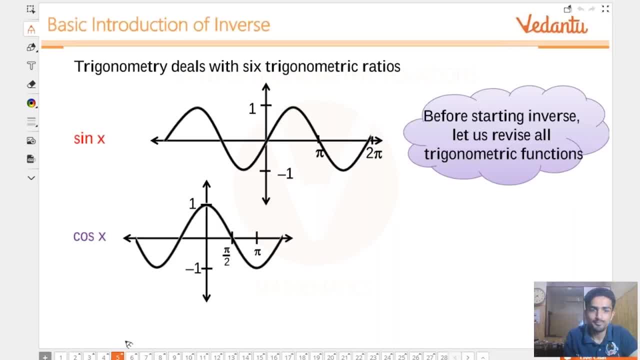 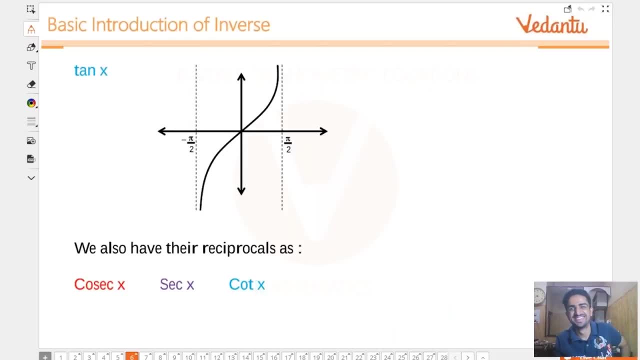 it is bit bit tough. okay now, this was a graph of 10. just keep it in mind. yes, Prathamesh, okay. similarly okay, Minag. now you need to keep in mind the graphs of cos and sec and cot also. uh, sine, cos, 10 are more important, but cos and sec and cot are like okay, if you remember good even. 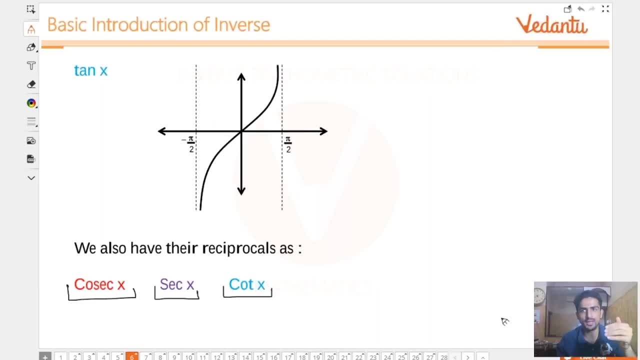 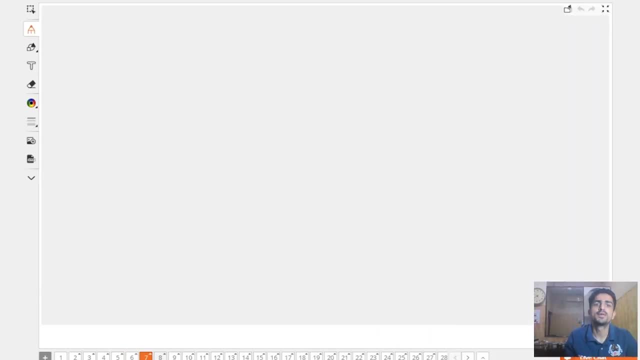 if you don't remember, that's fine, but sine cos 10, you have to remember these graphs. okay, now let us first start with inverse of sine. I hope no one of you will be thinking that we can write it like this. if any one of you is thinking like that, you know what you got to do. this is not. 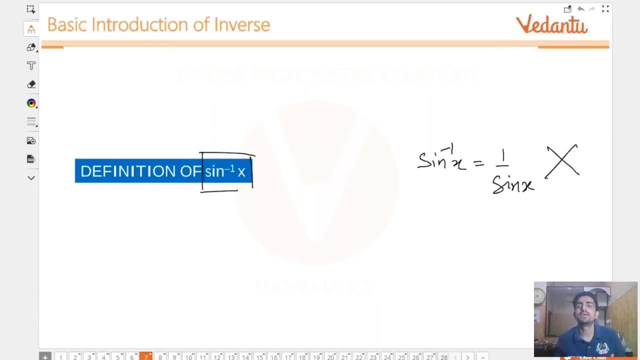 sine power minus one, it is sine inverse x, that is inverse of sine function. yes, don't worry. uh, just for little revision. yes, Austin, sine takes pi by six to half, then we know that sine inverse x will take half back to pi by six. sine of pi by six is half. sine inverse of half is pi by six. that is the definition or behavior of. 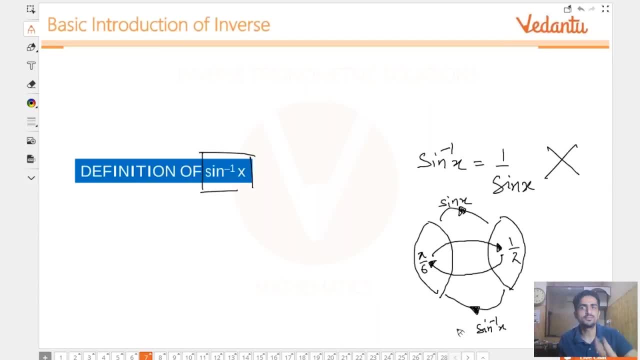 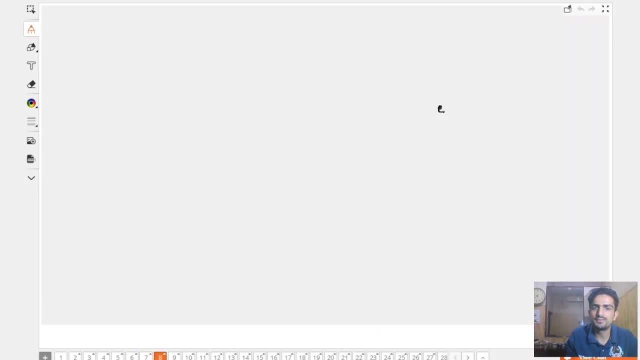 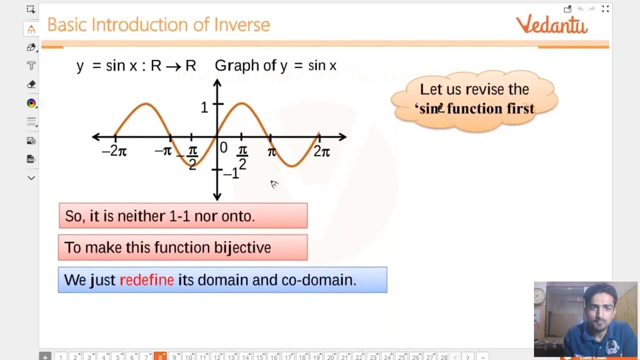 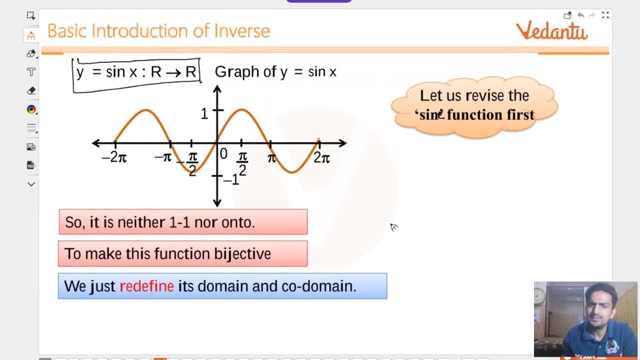 inverse function, and this is something we are going to study in this chapter. okay, so first of all, let me just prepare sine x to be invertible. listen guys, this is the graph of sine x, and when I consider it from r to r, this is clearly not one one and not onto. so we will actually change their domain. 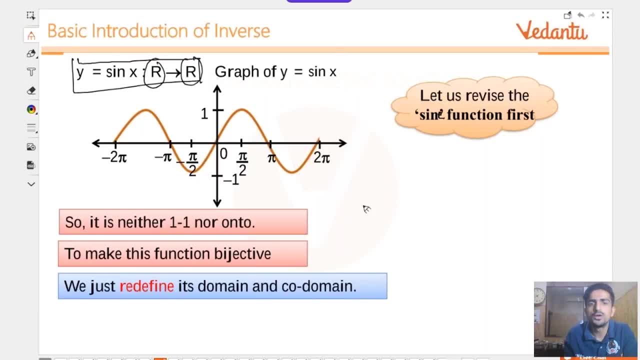 and co-domain. we will change these two things so that it becomes one one and onto- okay, this one. so I already told you that we will change it to minus 1 to 1 and my function will become onto. now just look carefully, if I change, take my domain to. 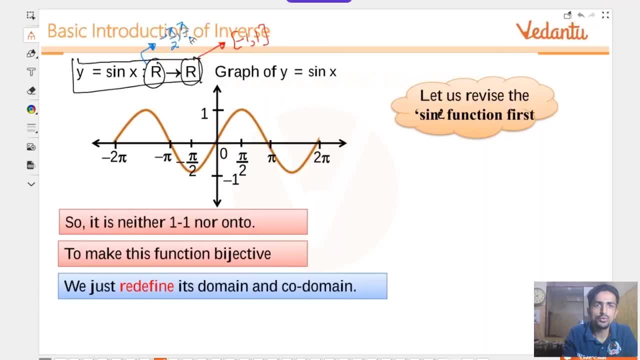 be minus pi by 2 to pi by 2, that is, I take these X to be my domain, then how the graph will look like, that is how it will look like this: much in minus pi by 2 to pi by 2. just see sine X is just increasing, increasing. 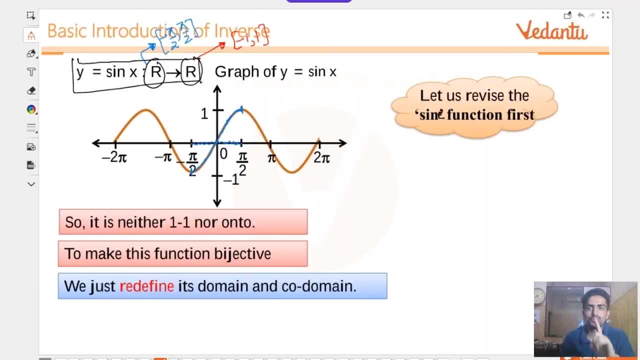 increasing, going up and up. so clearly it is 1: 1. so if I take my domain to be this and code main to be this, clearly my function is 1: 1. and onto normally students, they ask one, one question here, sir: why minus is pi by 2 to pi by 2, why not? 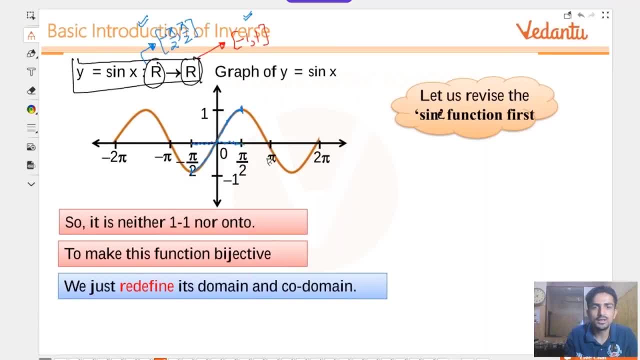 Anish, I was talking about the students like you. only, why not pi by 2 to pi? here also, function is 1: 1. yes, it is 1: 1. we could have taken that, but it was about defining it as one thing. we defined it minus pi by 2 to pi by 2. 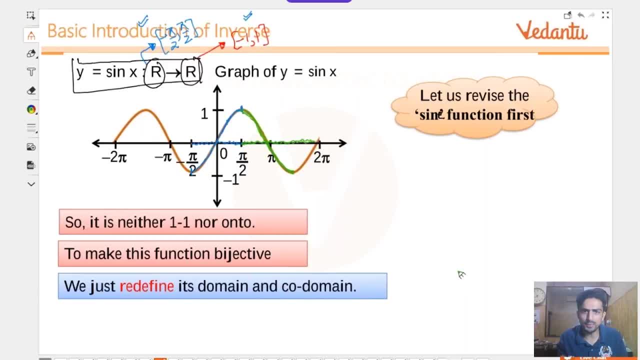 had they defined it from pi by 2 to pi, we would be studying it like that. ok, so it is like we had to define one thing. Karthikian, not at all. so we defined it from minus pi by 2 to pi by 2. so 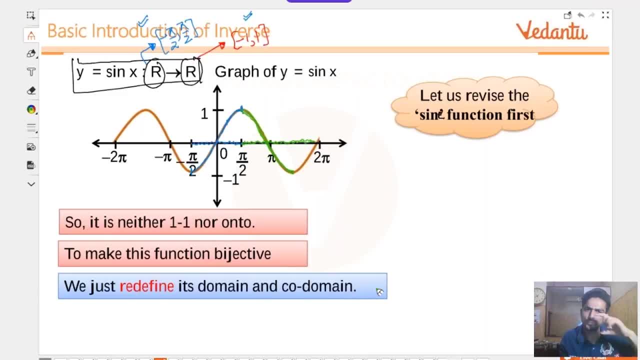 no special reasons or special theory about that. one branch is to be taken, that is taken from minus pi by 2 to pi by 2 taken. so that is convention. now we define for that only ok. so, guys, we define y equal to sine X as sine X from. 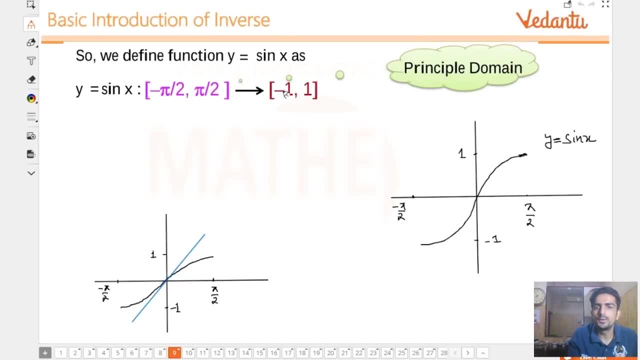 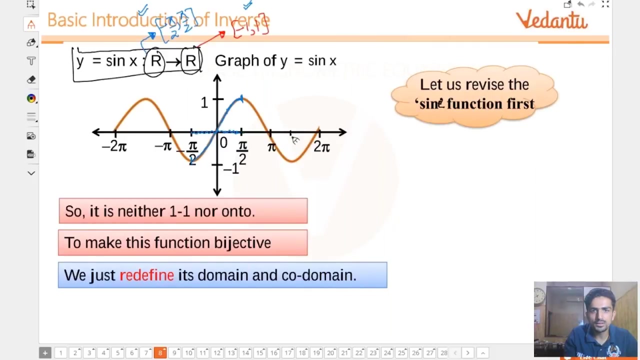 this domain to minus 1 to 1. for this domain and codomain, this function is invertible. very good by objective and hence invertible. Austin, better know the real value of sine X. so that about very well. from pi by 2 to pi 3. pi by 2, sorry from. 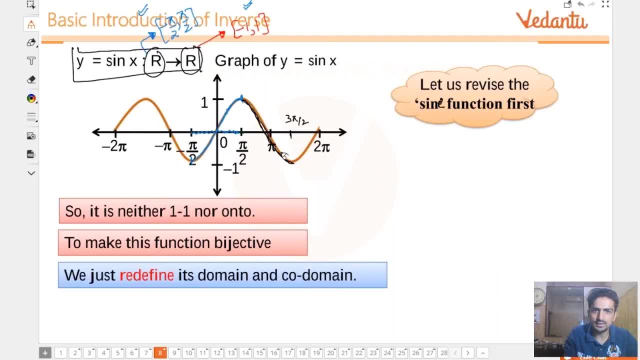 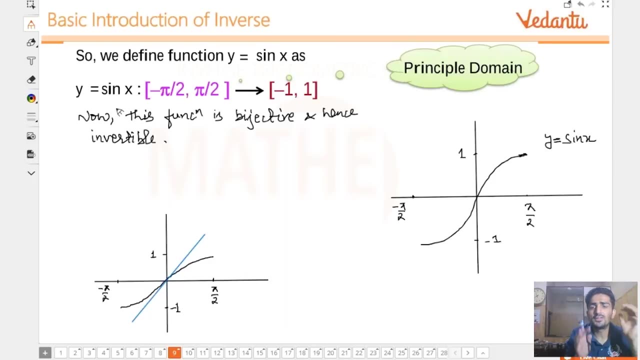 pi by 2 to 3, pi by 2 also, it is 1, 1. it is only decreasing, decreasing, decreasing. yes, Austin, there it is. so now, because now it x, now sine inverse x, will be a function from minus 1, 1, 2, minus pi by 2, pi by 2. 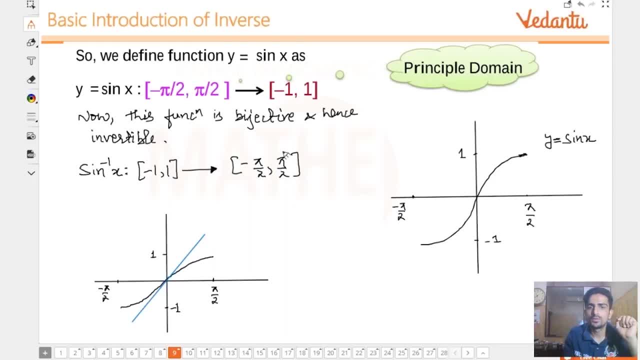 okay, now, before i just start with sine inverse, one thing you need to keep in mind is this: this new domain of sine x is equal to sine x, this new domain of sine x is equal to sine x, called principal domain of sin x, and you need to keep this principal domain in mind all the six. 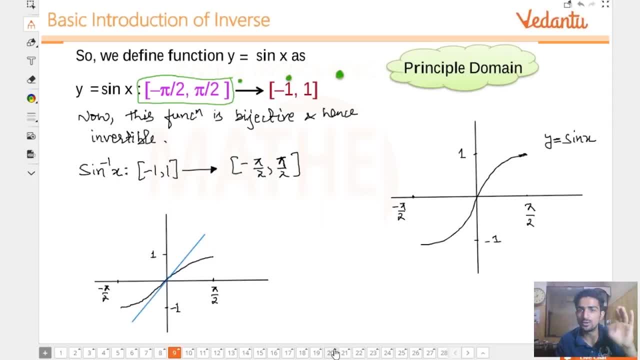 principal domains: sin x, cos x, tan, cot, secant, cosecant, all the six, for all six. you need to keep this principal domain in mind. this is very important. it will play a crucial role in many questions, especially in good objectives. so for sin x, it is minus pi by 2 to pi by 2. 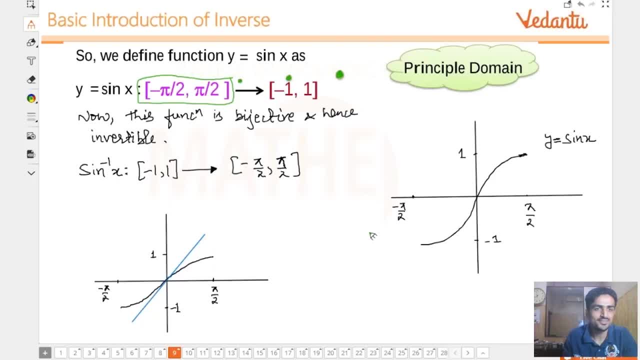 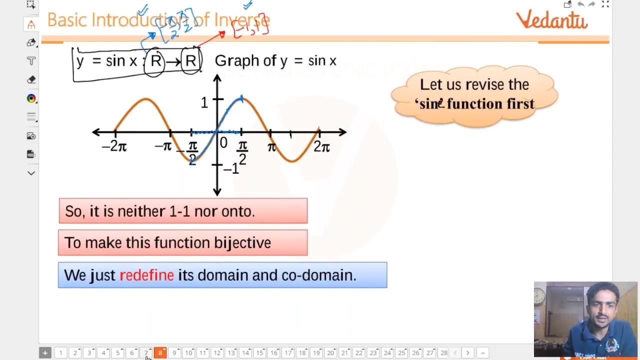 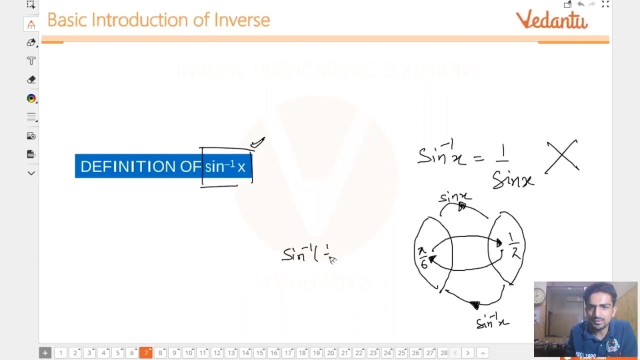 yes, now, before we doing we start with anything else, how to find values of sin inverse, as i just explained here. when somebody will ask me sin inverse half, i will just think it like that here to here: ok, sin inverse half is beta. wait, sin inverse half is that angle for which sin is half. 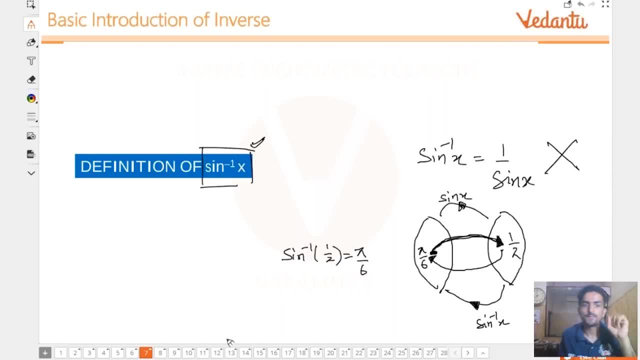 so it will be pi by 6. thats explaining the same thing from the graph. now, if this is x, this is y. sine takes X to Y and sine takes X to Y and sine takes X to Y and sine takes Y to Z. i don'tclock that x, i don'tclock it. 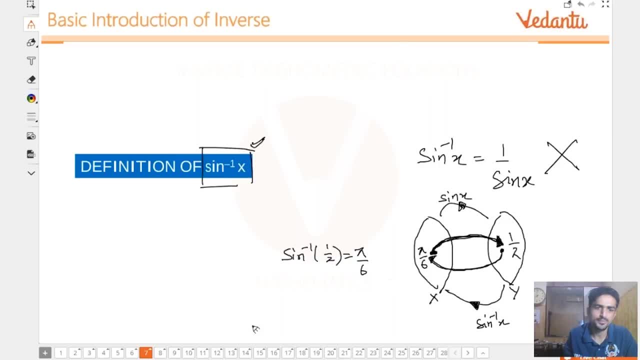 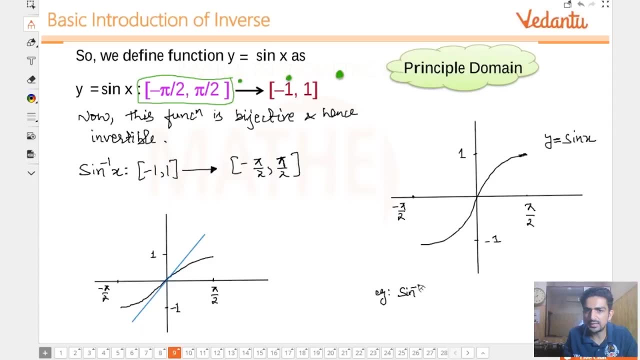 Sine inverse takes y to x. So here, if somebody asks me, Sir, sine inverse half, kya hai? Just look at the screen. I'll say half is somewhere here. Now I'm taking this on y, So sine inverse half will be somewhere here. 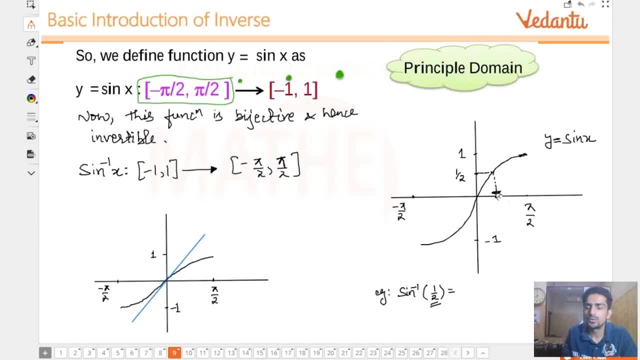 Now, which is this angle? Look at this like that. It is that angle for which sine is half. So when is sine half Pi by 6.. Okay, I'll give you one more example. Somebody asks me: Sir, sine of somewhere here. 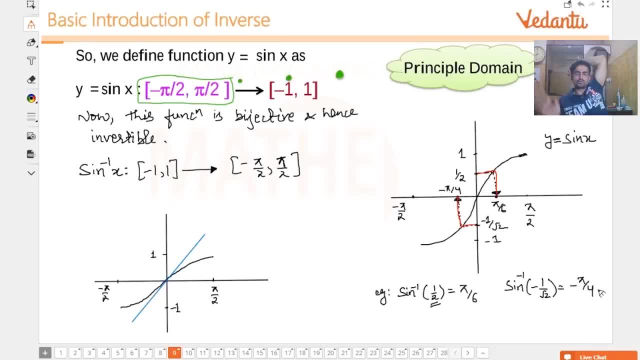 Nothing more than that, Melank, not now, After little time. First, just let me not deviate from the topic. Oh, Shagun, don't do that, beta, Beta. okay. let me just take one more example: sine inverse one. here is one. this is sine inverse one, the angle for which is sine. 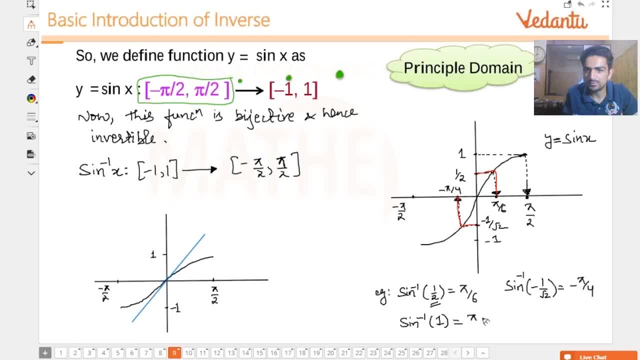 becomes one pi by two. that is all okay. before getting any much deeper into that thing, Sanmati as is, you don't okay, so they don't get confused with our okay. as such, it is not required. still, I'm giving you graph of sine inverse X. but believe me, 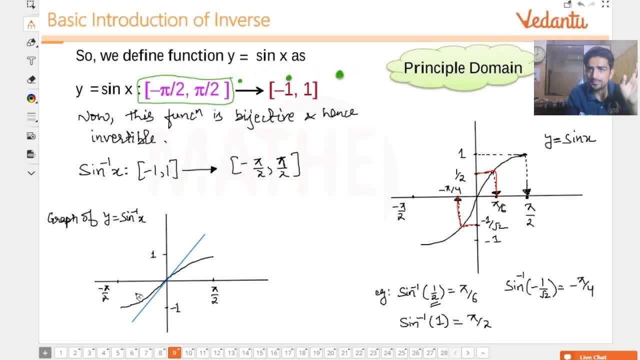 it will. you can see that it is not required, but believe me, it will not be used anywhere. okay, anywhere to not be used. but just for your reference, I'm giving you the graph, and graph is very simple. we know if we reflect the graph of Y equal to FX, about Y equal to X, like that. 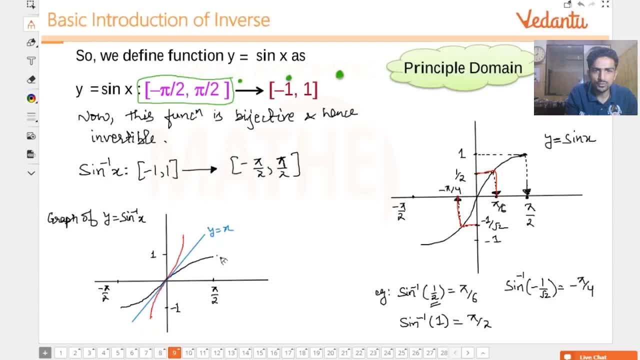 this is a reflection of Y equal to sine X about Y equal to X. then this graph will be Y equal to sine inverse X. that is how we draw the graph of inverse. we have done that in inverse functions. that graph of FX and F inverse X are nothing but reflection about Y equal to X. 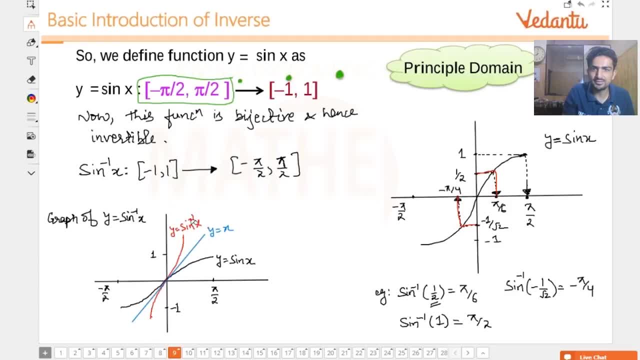 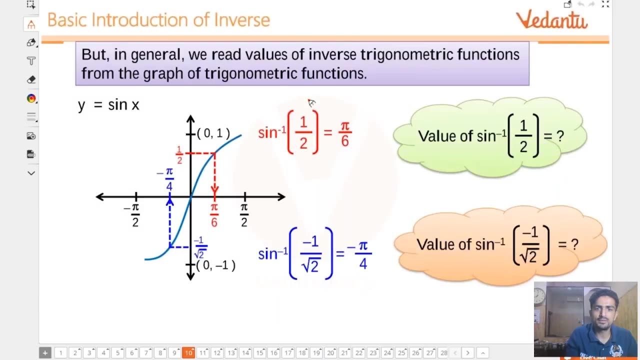 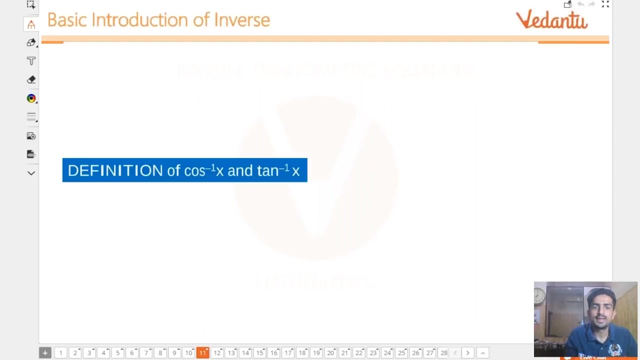 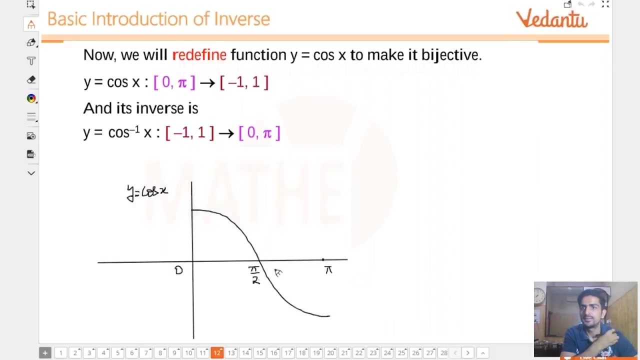 so that is how the graph of sine inverse X looks like, and it is no way required. just for your reference, I gave it to you few more examples. primarily they are same. next is cause inverse X. okay, now we will redefine cause X. obviously. now, this is a. 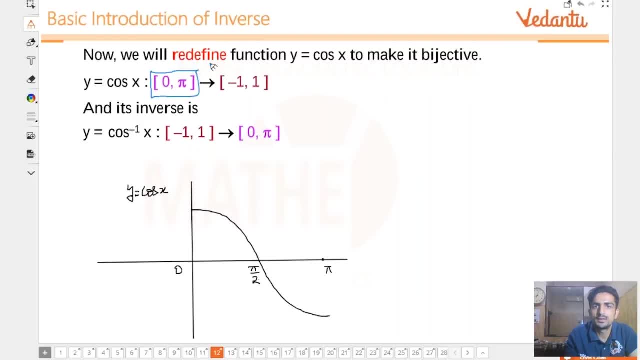 new domain of cause X, which we call principal domain. so cause X principal domain is 0 to PI. you need to remember that. I'll be asking these things in next class, okay. so principal domain of cause X is 0 to PI and this is code mean minus 1 to 1. this is a graph of cause X in 0 to PI. clearly, 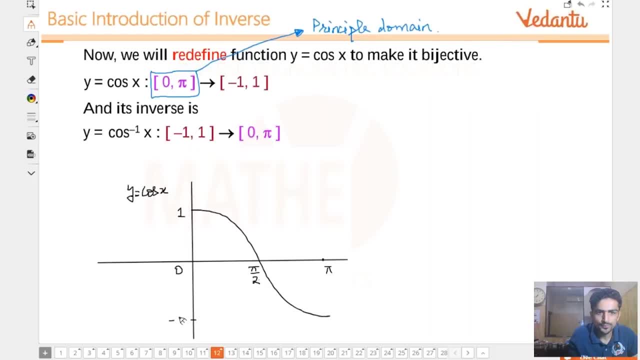 it is 1, 1 and on 2, so it is invertible and cause inverse will be minus 1. 1 to 0 to PI. if F is from A to B, F inverse is from B to A. now if we say what is cause inverse, half we 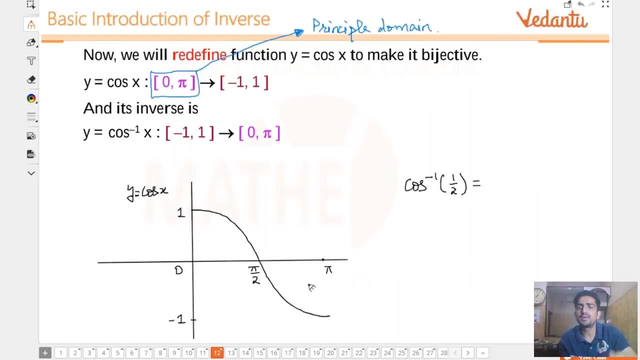 have to begin with. always try to like, plot the graph and find the values, as I am doing. I'm telling you it will be helpful. okay, in the beginning, do this only so. here will be somewhere half this angle. try to understand. I am saying this angle cause. 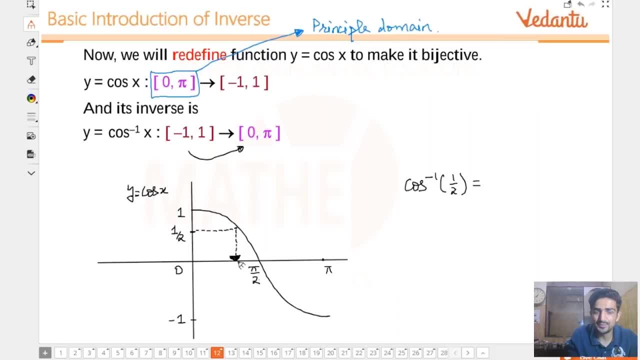 inverse key output will be an angle. so this angle we require now. I think of this angle as this is that angle for which cause becomes half. now, when does cause become half at PI by 3? so how will you think about cause inverse half? it is that angle for which cause becomes half. 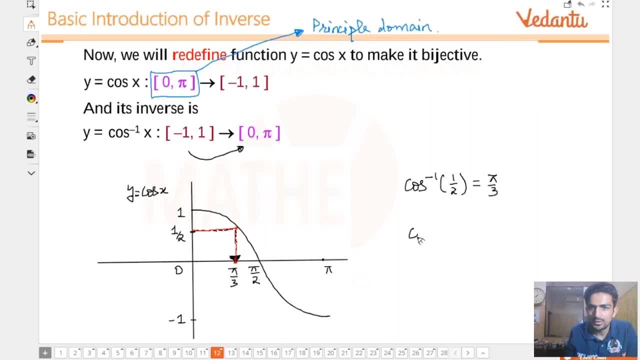 now, if somebody asks me cause inverse minus half now from the graph- just try to see from the graph I am getting that- my answer is an angle in PI by two to PI first of all, as we did in the beginning also. Now, what is this angle? Just listen to my words carefully. It is that angle for which cos becomes minus half. Now, for which angle cos is minus half, Supplementary of pi by 3. That is 2 pi by 3.. 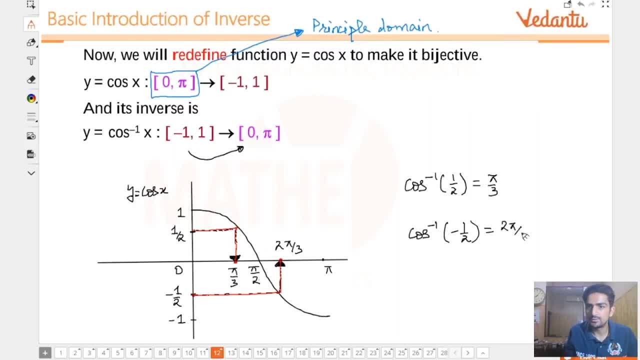 Very good guys. Now it is very important guys, I am going to tell you one thing very important. You need to understand that cos inverse of anything negative it will lie in pi by 2 to pi. It will lie in pi by 2 to pi, Because that is the codemain of cos, Cos inverse. Codemain of cos inverse is 0 to pi. only, You cannot go beyond 0. You cannot go ahead of pi.